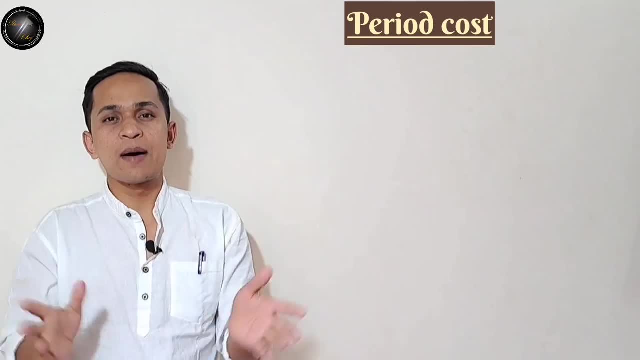 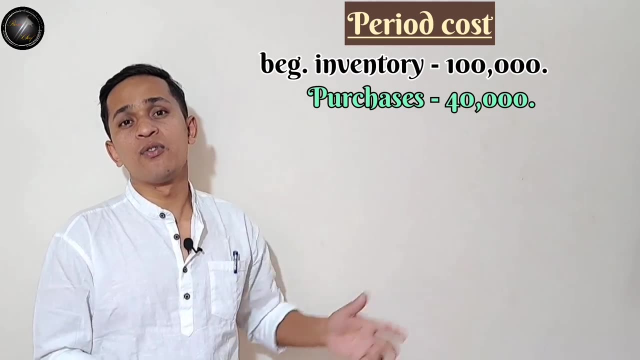 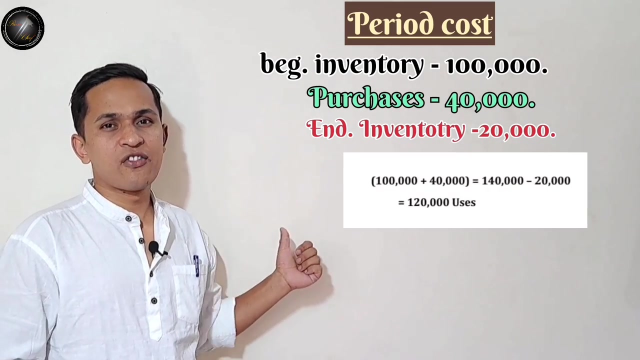 percentage, our food cost percentage. Okay, for example, our October beginning inventory was 1 lakh rupees and we purchases 40,000 rupees in our food in October and our October ending inventory is 20,000.. It means 1 lakh 40,000 minus 20,000.. 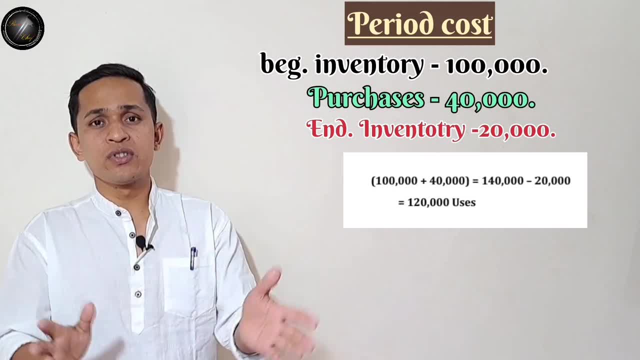 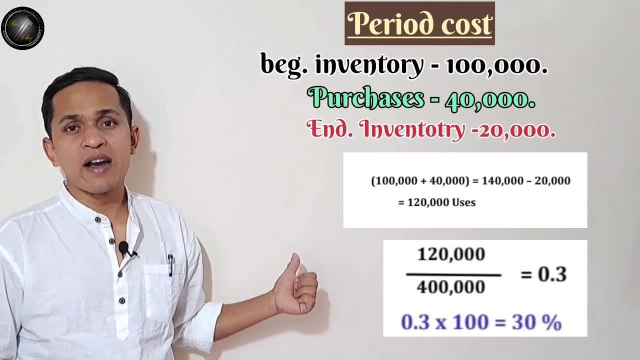 is equal to usage. It means we used 1 lakh 20,000 in our food in October. Okay, now we take the usage and divided by our food sales, which is 4 lakhs rupees, 1 lakh 20,000 divided by 4 lakh is equal to. 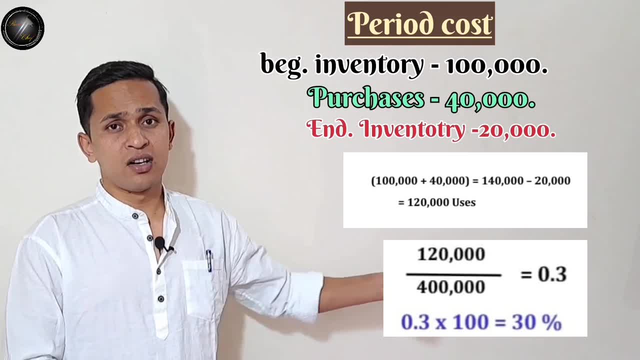 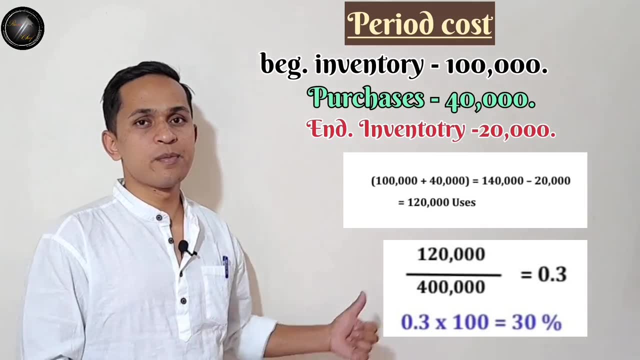 0.3 its Cox. now take the Cox and multiply it by 100 is equal to Cox percentage. It means our food cost percentage is 30%. Okay, I hope you understand how to calculate pallet cost and period cost. 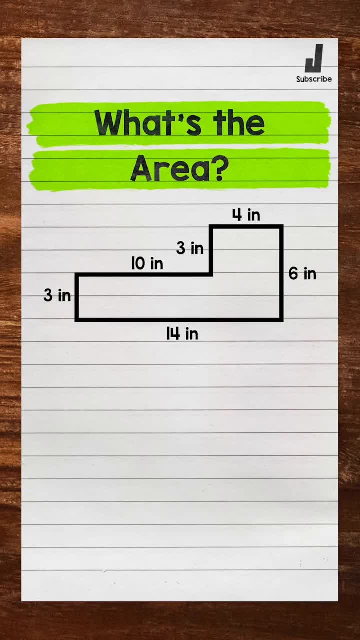 This is math with Mr J. Let's find the area of this figure. We first need to separate it into simpler shapes. For example, we can split this figure right here. So we have two sections, section A and section B. We need to find the area of those sections and then add them for. 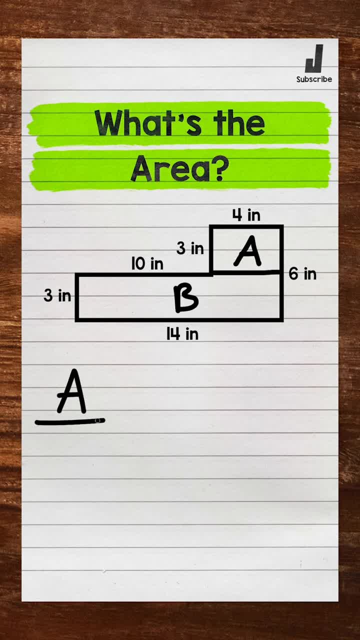 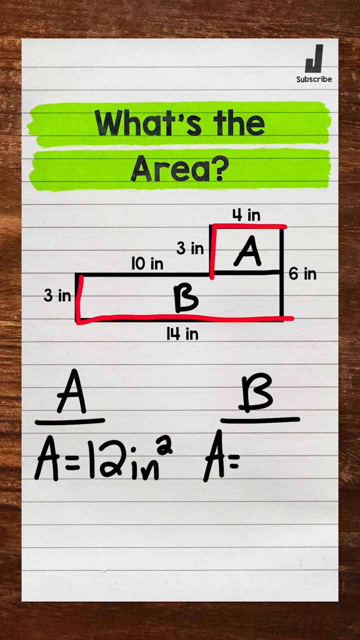 the total area. Let's start with section A. We have a four by three rectangle. Four times three is 12.. That means the area of section A is 12 square inches. Now we need the area of section B. We have a 14 by three rectangle. 14 times three is 42. So the area of section B is 42. 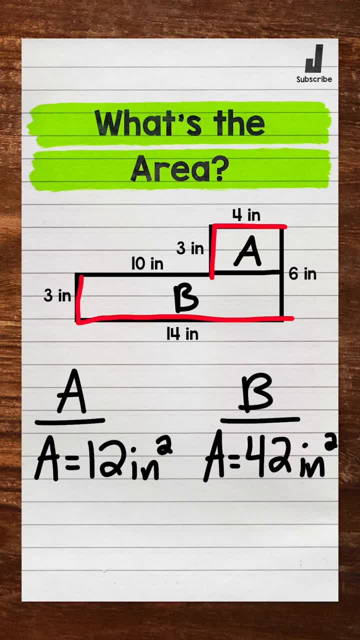 square inches. Now we add those areas for the total area of the composite figure, 12 plus 42 is 54.. So the total area of the composite figure is 42.. total area is 54 square inches. Until next time, peace.